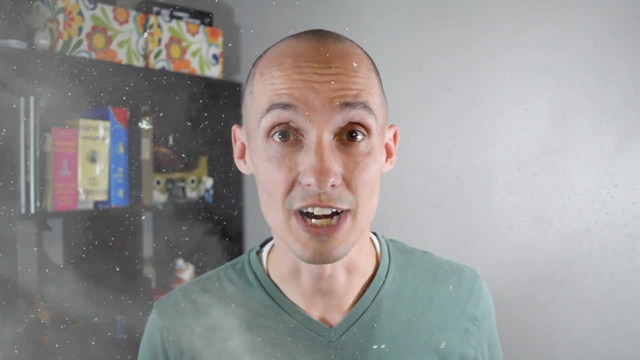 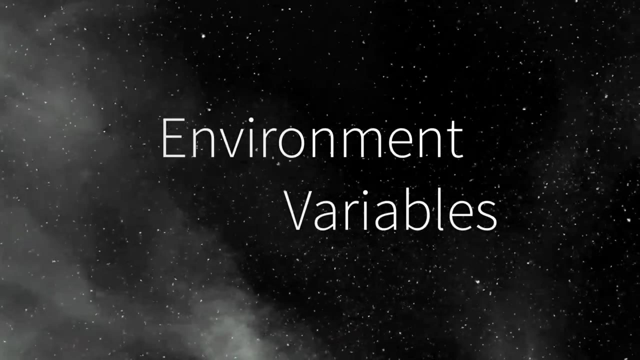 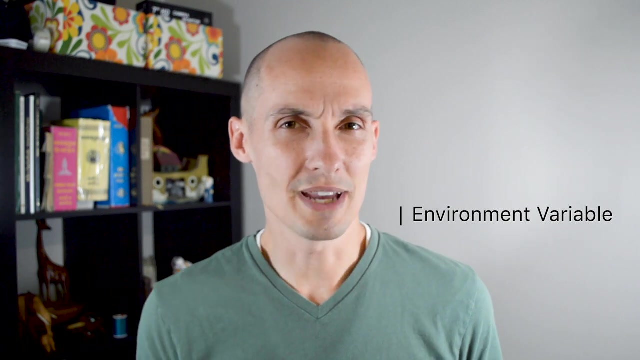 Today we're talking about the environment, Not that environment, your program's environment. In my last video I mentioned an environment variable And after filming it occurred to me that some of you may not know what in the world I'm talking about. Now, this could be a beginner. 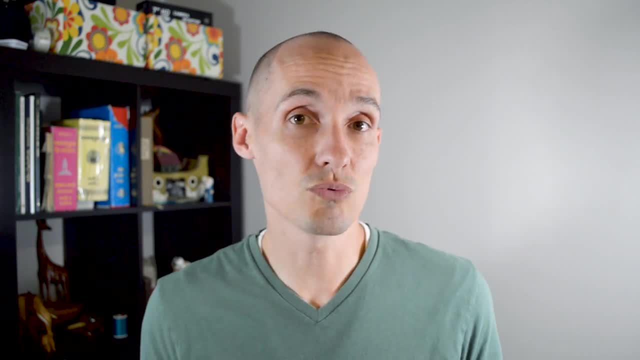 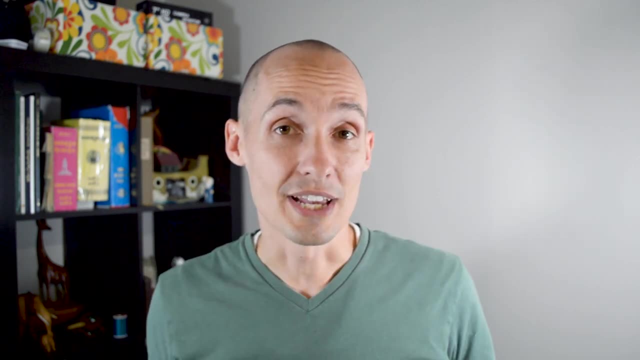 topic, but I've also met a lot of juniors and seniors who don't really understand how environment variables work and don't really have a lot of experience with them. So we're just going to say this is an everybody topic today. Okay, so to start, get out your terminal, So open up a 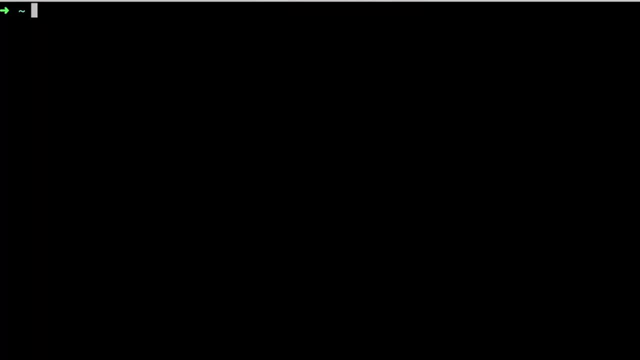 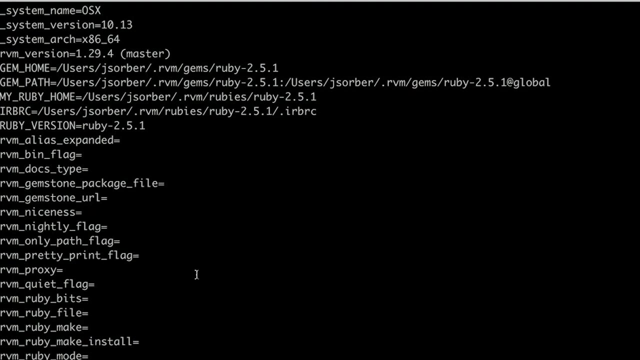 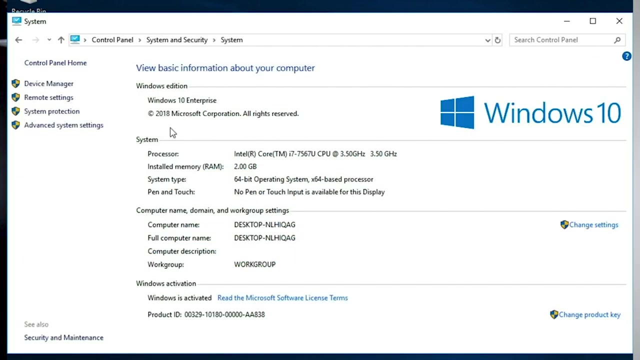 terminal. If you're on Linux, macOS or any other Unix-style OS, just type env. Now this is going to print out a bunch of variables. This is what we refer to as the environment. If you're on Windows, it's a little trickier: Go to the control panel, click here, click here and here and then. 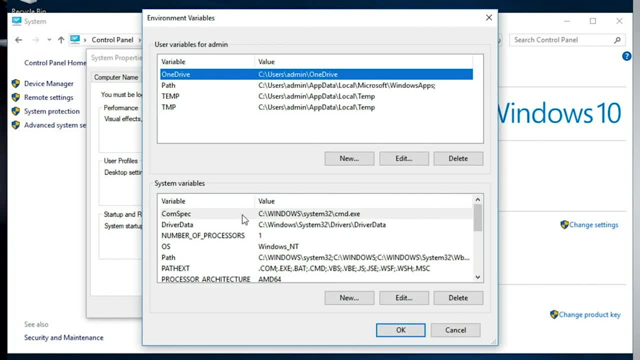 down here at the bottom, click there. You know it's almost like Microsoft Word. Microsoft doesn't want you to know that there are environment variables there, But they're really there. Everybody has environment variables, So each variable has a name and a value By. 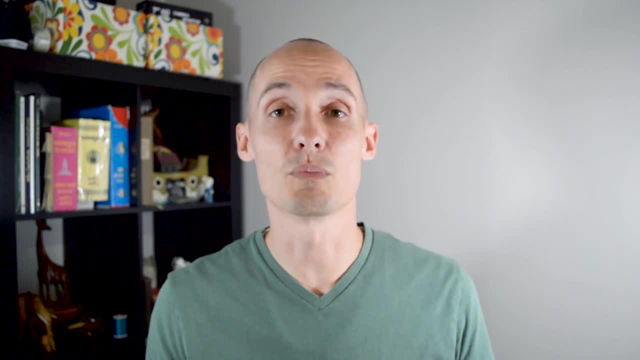 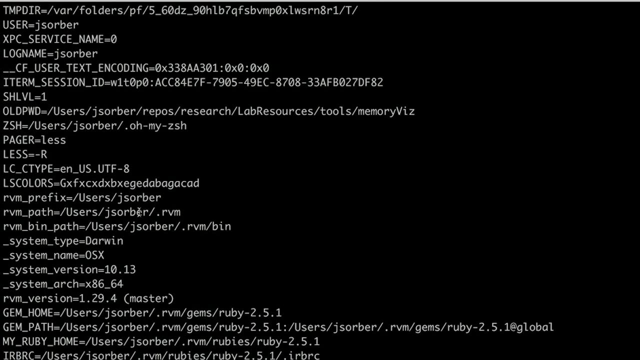 convention. the names are all uppercase. They don't have to be. Of course you can name them whatever you want, but why confuse people? And the values are strings. They really can be anything you want them to be, And the point of these variables is to communicate to programs how the 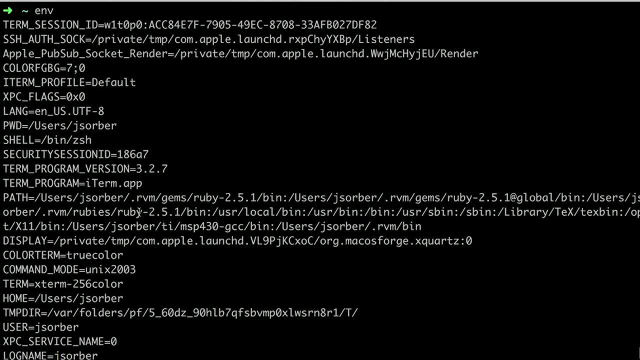 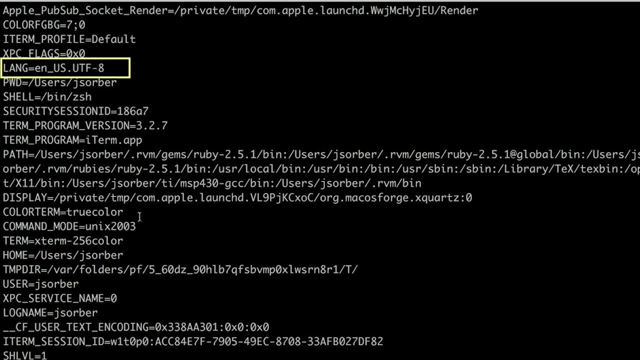 machine is set up and sometimes to control the behavior of programs. So, for example, in my environment it tells me that I'm going to be able to control the behavior of programs. So it tells my programs what users logged in and what my home directory is and what language I'm. 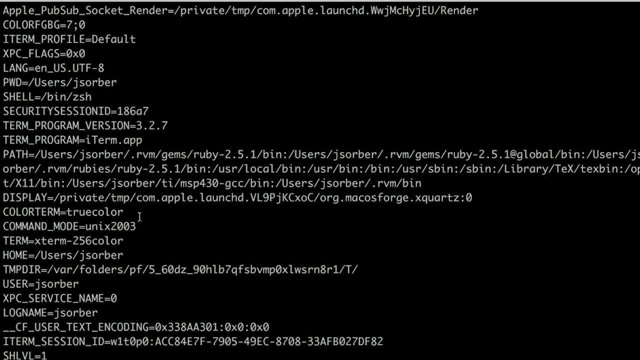 currently using and a lot of other things. So one useful variable is the path variable. This one tells my computer where to look for executable programs, And if I put my program in any of these directories, I can run it from anywhere without typing the path to the program, And that's why I 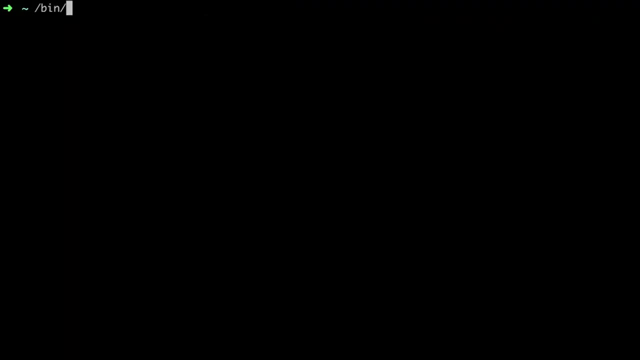 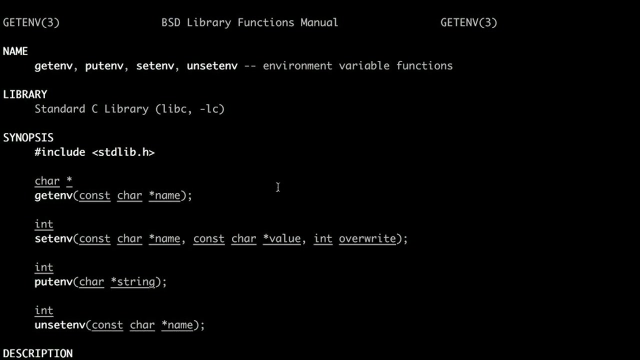 can just type ls and I don't have to type out the path to the binary like this, Though of course that definitely works too. If a C program wants to read an environment variable, then it can use the getenv function. Just pass in the variable name you want. You'll get null if it isn't set, and a. 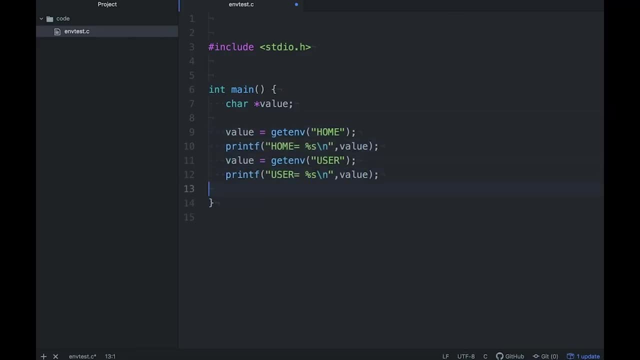 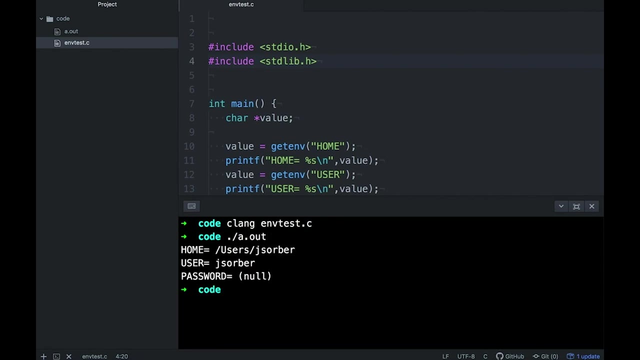 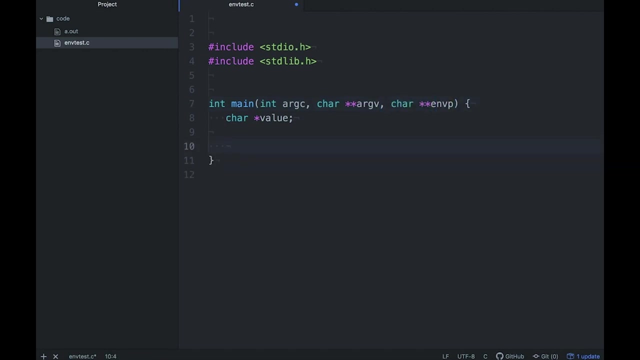 pointer to the value, if it is Okay here. So let's print out a few that are set and one that isn't, So you can see how this works and compile it and run it Easy. And now, because we need at least two ways to do everything, we can also rewrite main like this: Now, most of you have 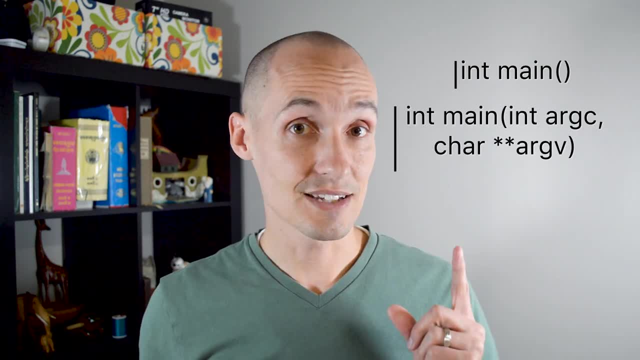 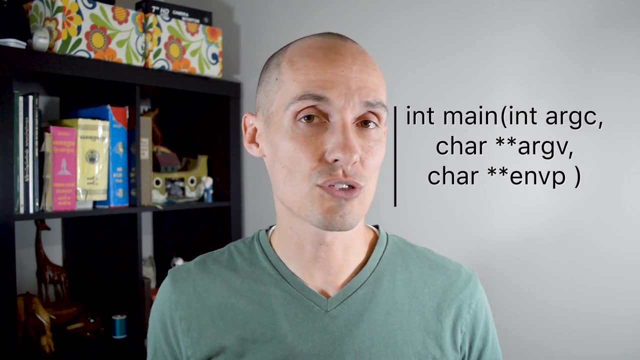 seen main look like this and like this with argc and argv. Many of you may not have seen this, but I've seen it look like this. But this is also supported on most platforms. And that third argument: envp is actually the environment. This is a list of environment variables. It's really a 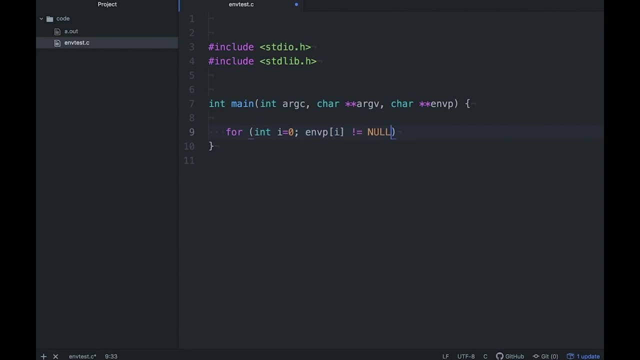 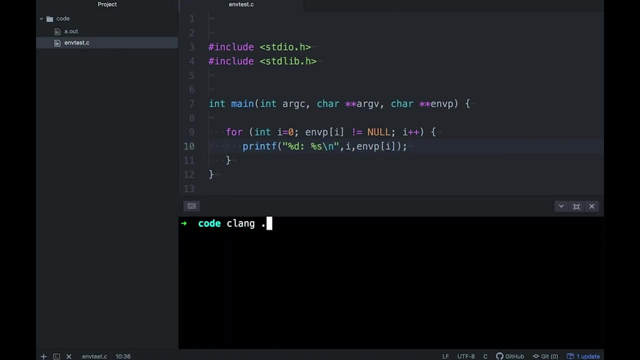 list of strings, And I don't know how long it is, but it's null terminated, So I can just loop through the array printing out the variables until I get to a null pointer. And so let's compile it. We run it Great, Easy And, of course, because we need at least three ways to do. 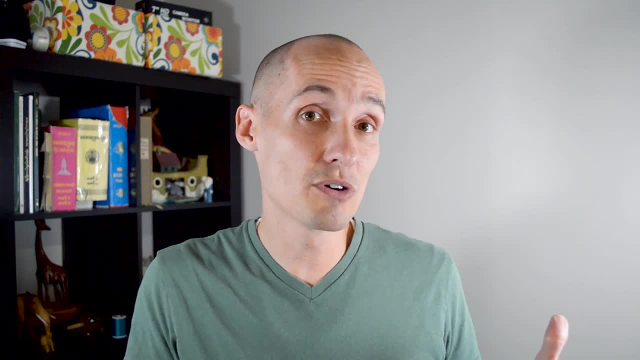 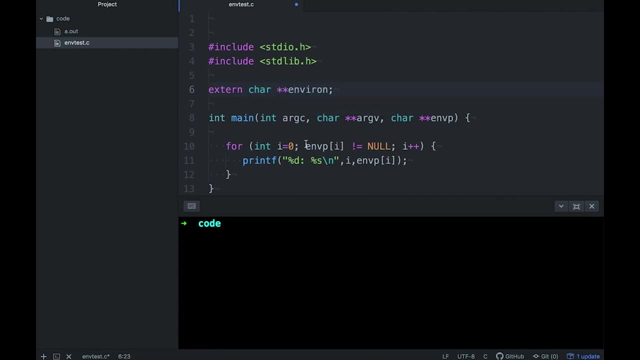 everything. I'm not kidding, I'm serious. And we can also do this with a variable called environ. that is a pointer to the list of environment variables. So we define it as extern because it's actually defined elsewhere in libc And we can loop through that array just like we did the envp array, And we just get the same. 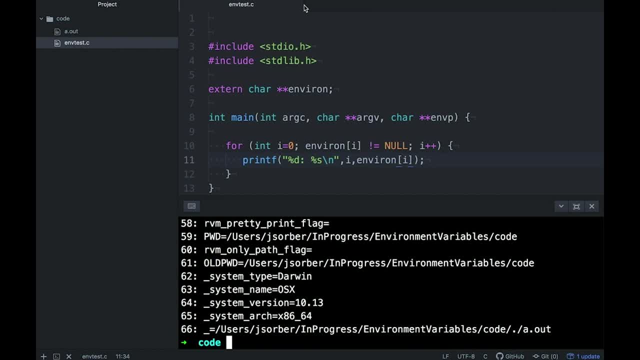 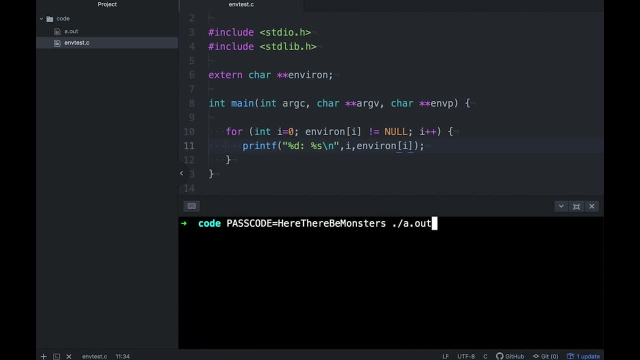 results: See Okay. so now say I wanted to set an environment variable. If I'm in the terminal I can just set it on the command line before I run a program. This will set the variable just for that program. Now let's say I want to set it for the entire environment And I can just set it. 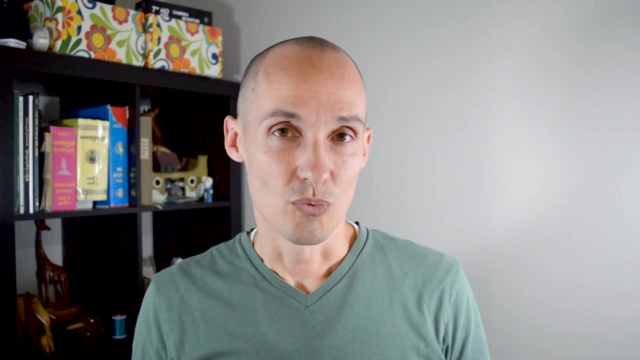 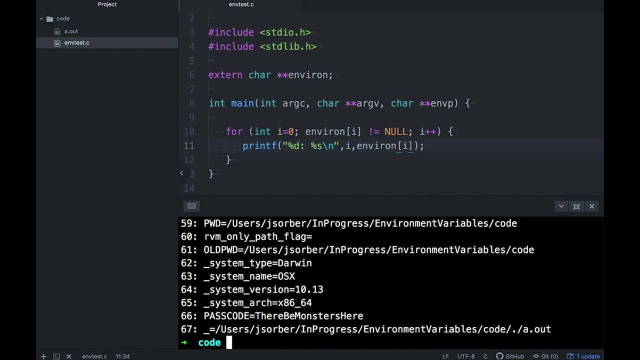 for the entire terminal session. Then I use export. Why is it called export, you ask? No idea, but now the variable will be set for every program that runs in that terminal session. And of course I can use the unset command to unset the variable if I decided that my use of export was a bit hasty. 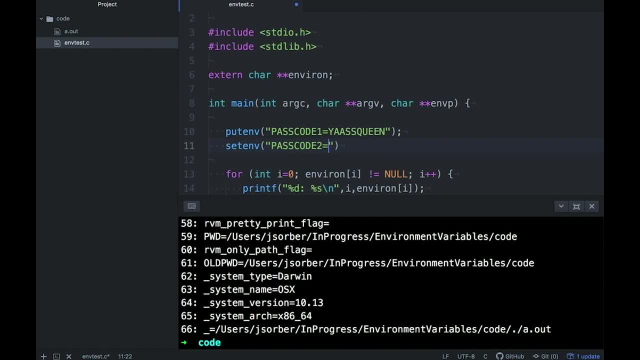 And if I'm inside my program, I can set a variable using setenv or putenv. Both do roughly the same thing, they're just called slightly differently. Now keep in mind that this just sets the variable for this setenv on the program. 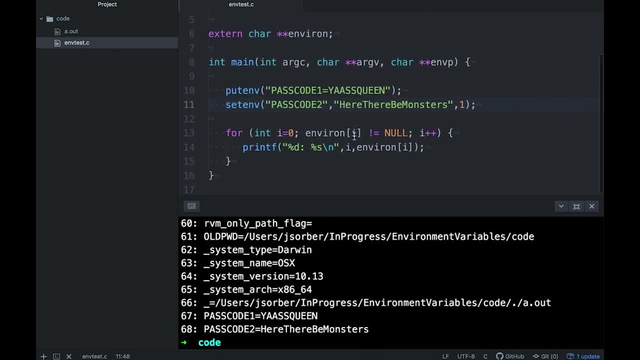 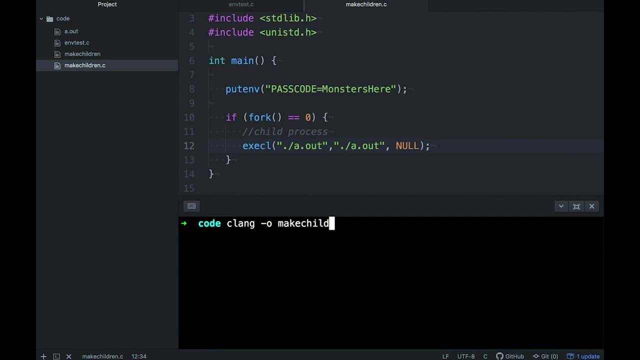 program and any child processes that it creates. After this program runs and we go back to the terminal, that variable will not be set. But if my program creates a new program, if it forks off a child process or executes a new program, then that child will see the variable change And that's pretty much all I.